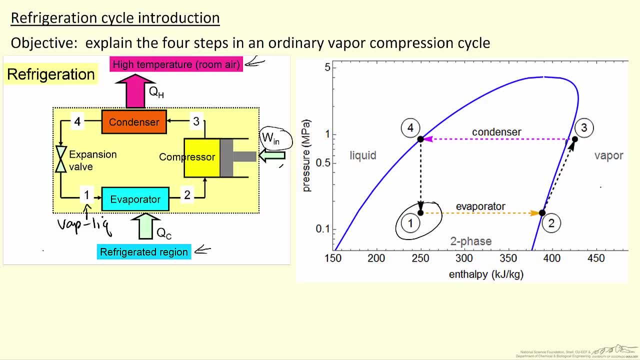 for this refrigerant being used. R134A. this is about minus 20 degrees C, So the refrigerated region has to be a higher temperature than that. We transfer heat and we evaporate the refrigerant. to this point We have a saturated region. 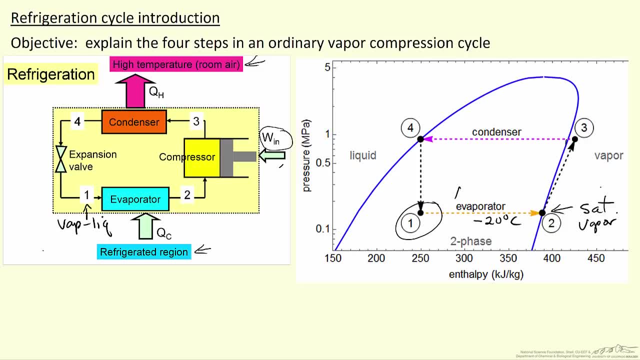 We can write an energy balance for this step and it says delta H is equal to QC. We now take this saturated vapor and we use a compressor, so we put work into the system and we use a compressor to raise the pressure from low pressure to higher pressure, in this case. 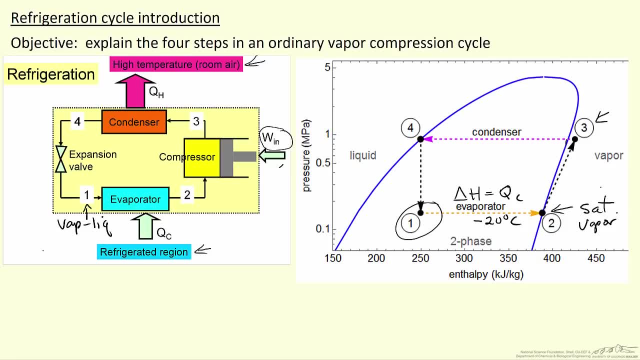 we have increased the pressure from 0.15 megapascals to about 0.9 megapascals, And so the energy balance for this step is delta. H is equal to W, So this step is assumed to be adiabatic. 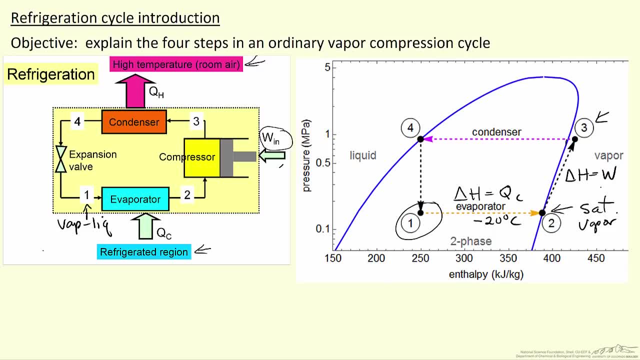 To increase the pressure of a gas, we have to also increase the temperature, because we're putting work into the gas. The next step, going from three to four, we're going to take this higher temperature and higher pressure vapor and we're going to condense it to a liquid at constant pressure. 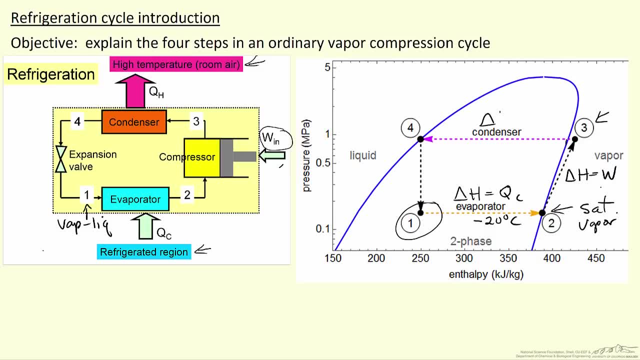 So this step is constant pressure. Energy balance is now delta H is equal to QH. Removing heat here, transferring it, for example, to the back of a refrigerator to condense to a liquid at high pressure. This high pressure liquid, then we expand through a throttle, an expansion valve, and 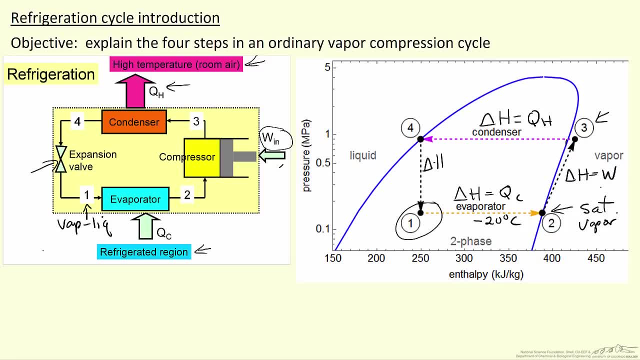 the energy balance for this step is that delta H is equal to Z, And that's the energy balance for this step. Assume it's adiabatic, because it's rapid, there's no work being done. But when we lower the pressure of a saturated liquid, the liquid evaporates. 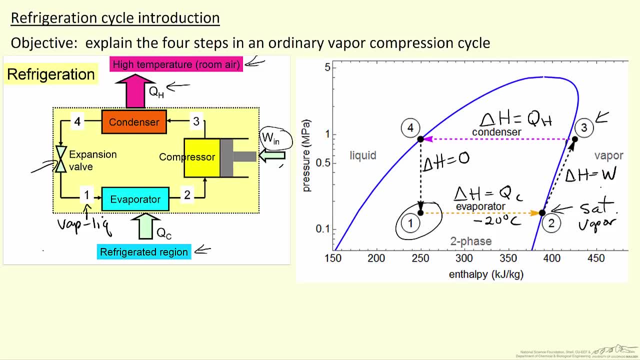 Because it's adiabatic. the energy to evaporate it comes from cooling everything down. This is how we get the low temperature that we need to accomplish our refrigeration, And so the overall cycle is the running this refrigerant through an evaporator at low pressure.